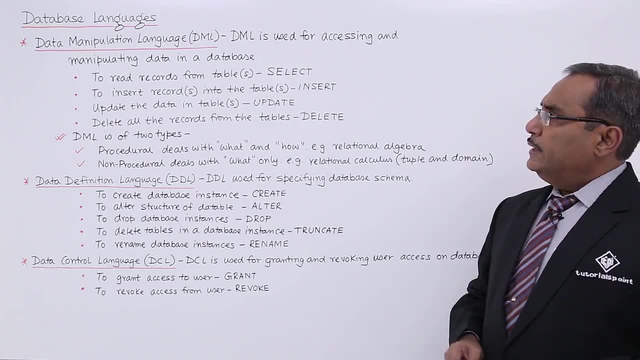 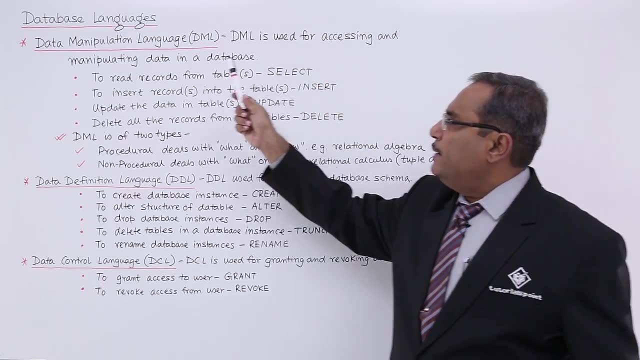 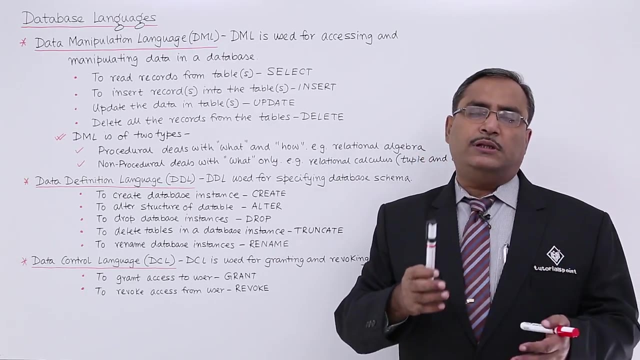 we are going to discuss data manipulation language, Data manipulation language. in short it will be called as DML. DML is used for accessing and manipulating data in a database. That means to read from the data and do some manipulations on that particular data. we require the data manipulation language, So let me go for some. 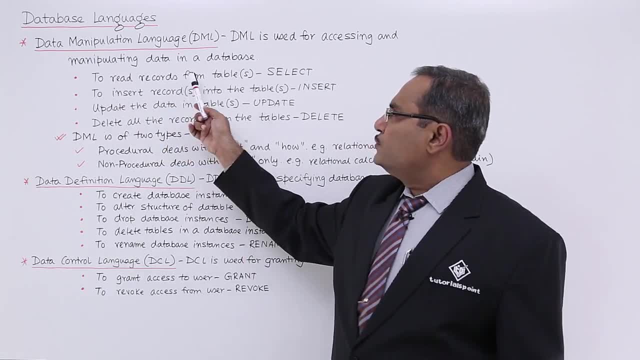 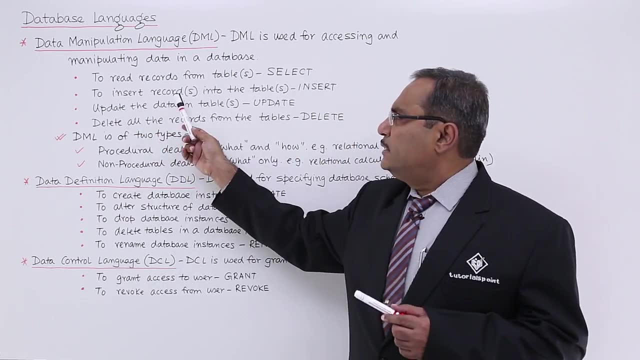 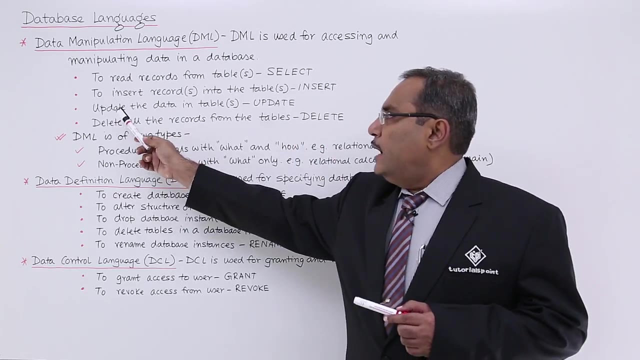 ideas, some examples, rather, To read records from the tables, here we usually use the keyword, that is a select, To insert records into the table. So here the keywords will be: the command will be: insert: Update the data in the tables. Here the command will be: update, Delete. 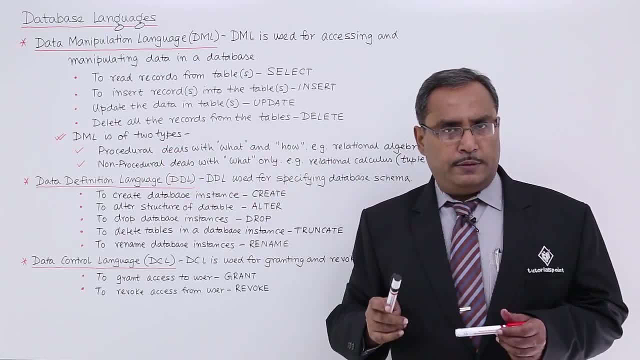 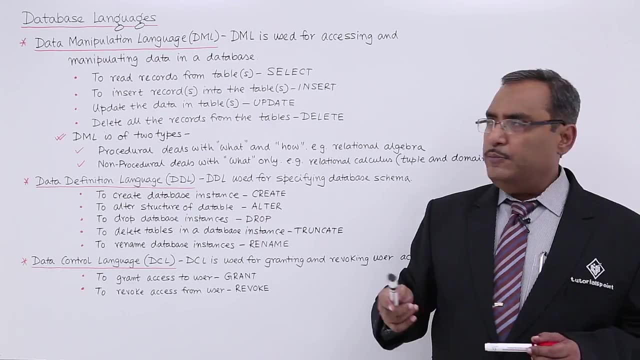 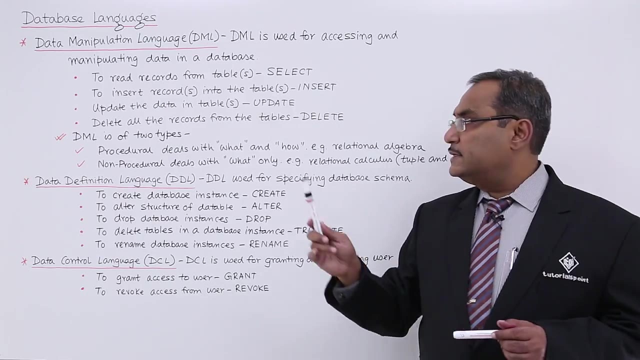 all the records from the tables and the command will be delete. It is obviously not mandatory that. obviously we are not going to delete all the records for each and every time. Also, you can go for a selective record deletion from the database. So for both the cases, the command will be delete. This is. 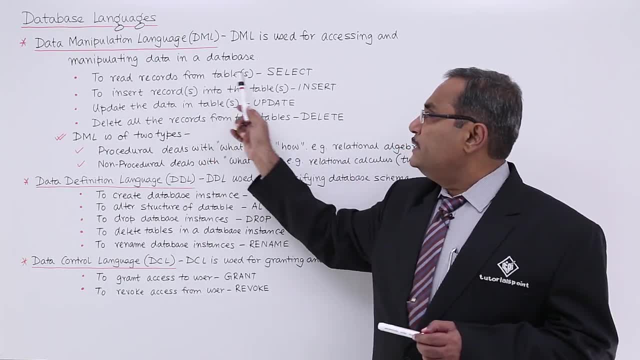 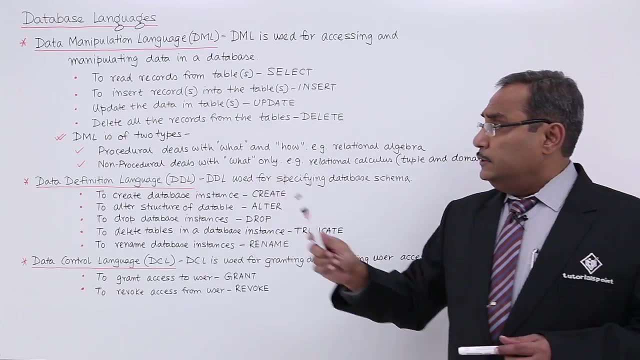 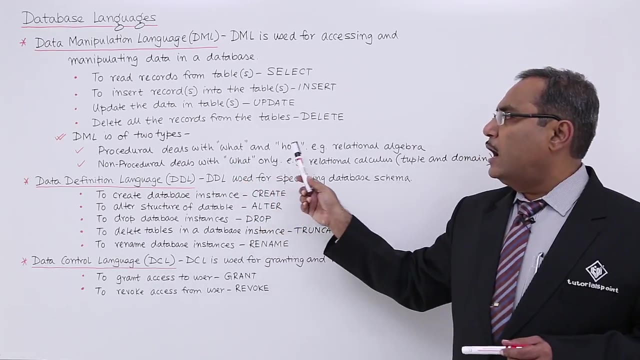 the keyword and this is the command. So we are having this: select, insert, update and delete. These operations can be done in our DML. This DML can be of two types. One is your procedural, which deals with what and how. So procedural query language deals with what That means, what 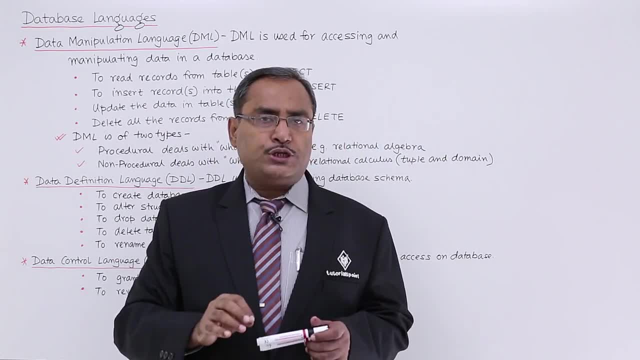 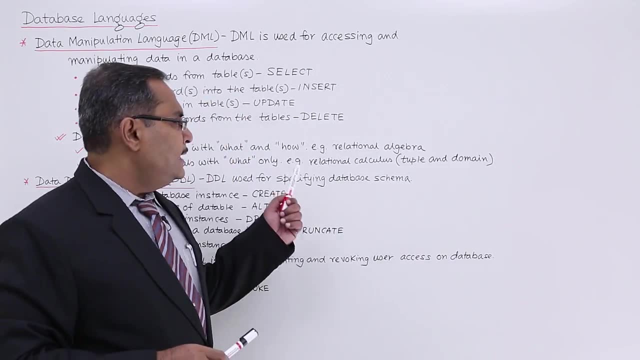 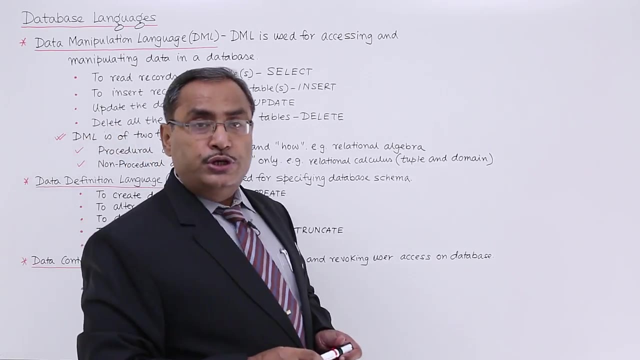 has to be done And how. that means how that operation will be executed. you should have to write that one in the respective DML statements And as an example we can go for this relational algebra. So relational algebra is an example of procedural query language. 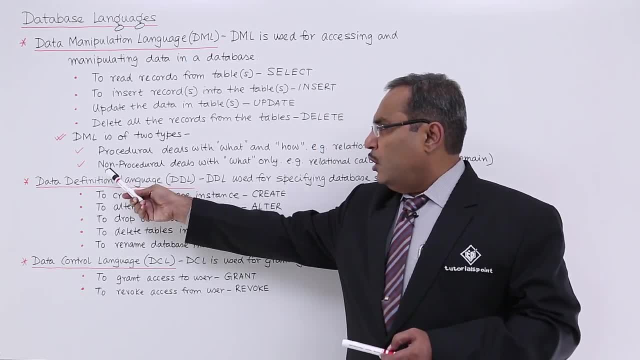 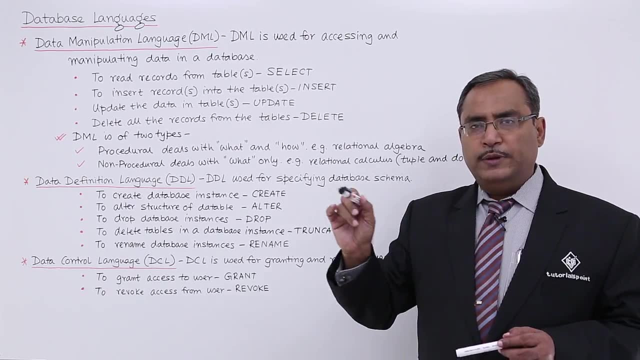 procedural DML query language. In case of non-procedural, it deals with what? only what. It deals with what That means. you are supposed to write that one in a respective syntax, So you need not to bother for the how the query is getting executed. 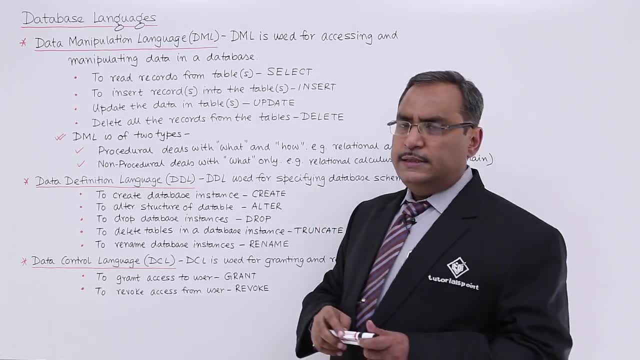 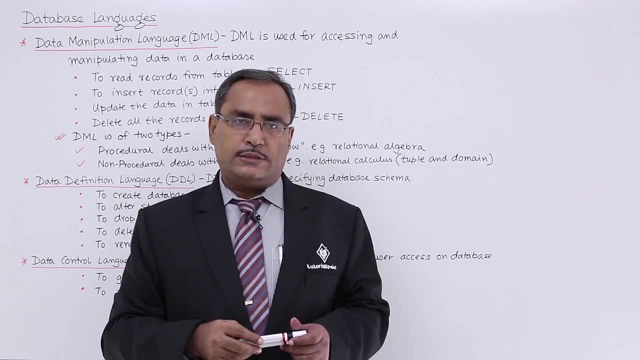 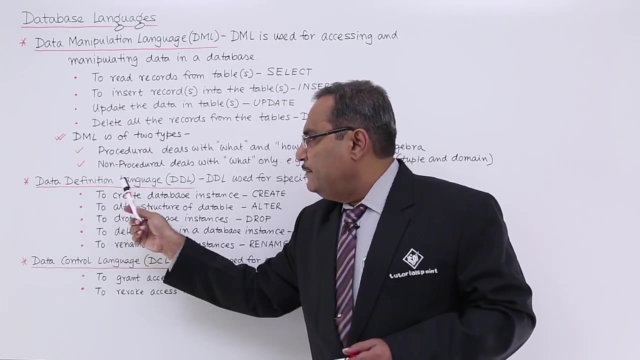 And, as an example, you can go for relational calculus. This relational calculus can be of two types: One is a domain relational calculus and the other one is a tuple relational calculus. So this is the DMA classification, DML classifications. We are going for data definition language. Now that is my DDL. DDL is used for specifying database. 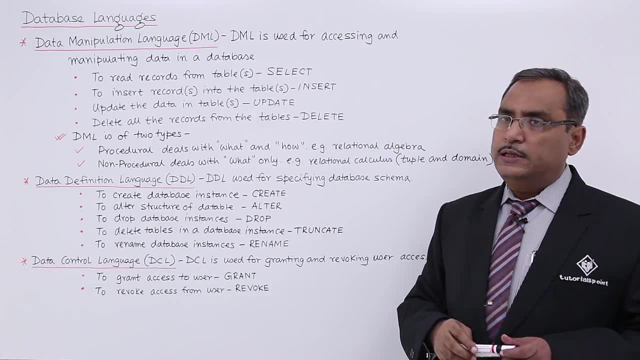 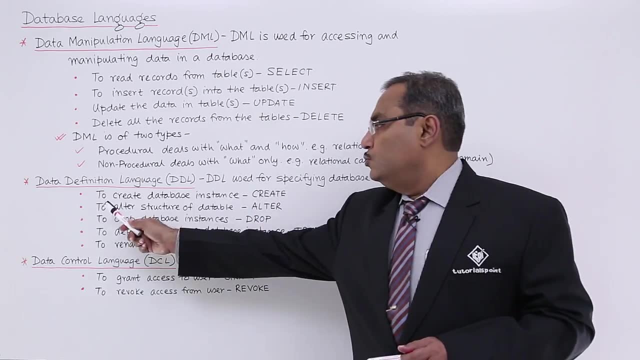 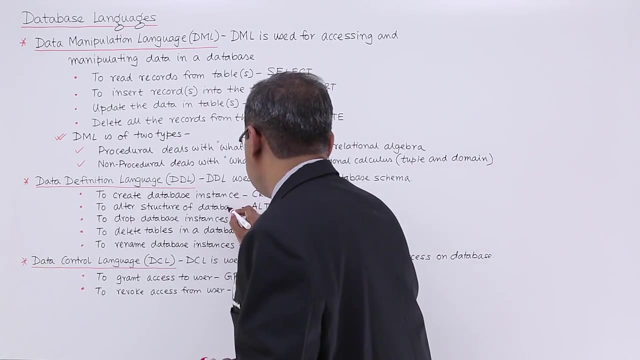 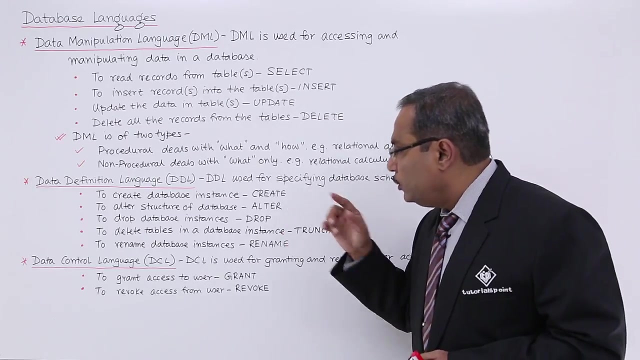 schema. So to define the schema we require this DDL To create database. instance command will be create To alter the structure of database. let me make it database To alter the structure of the database. so the command will be altered To drop database. 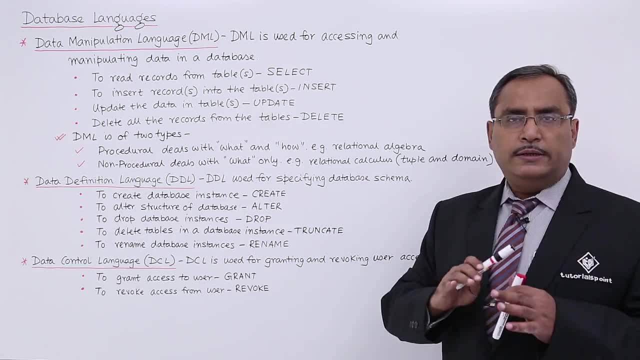 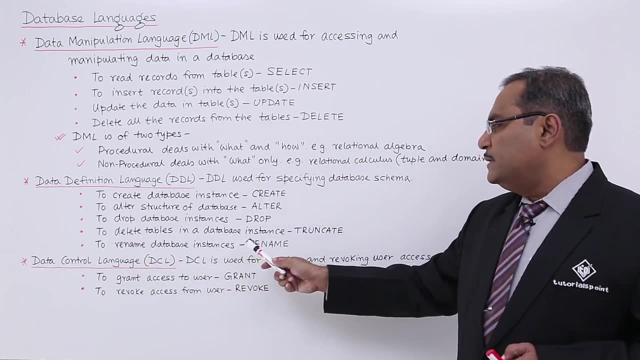 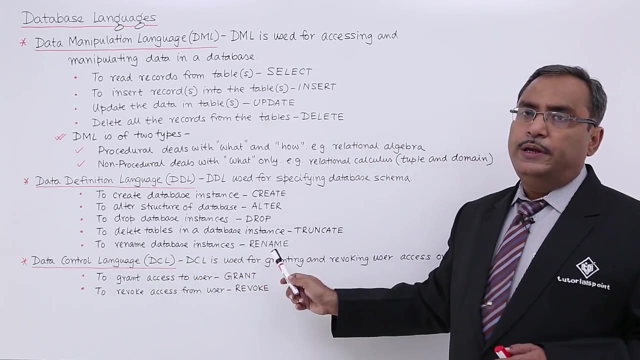 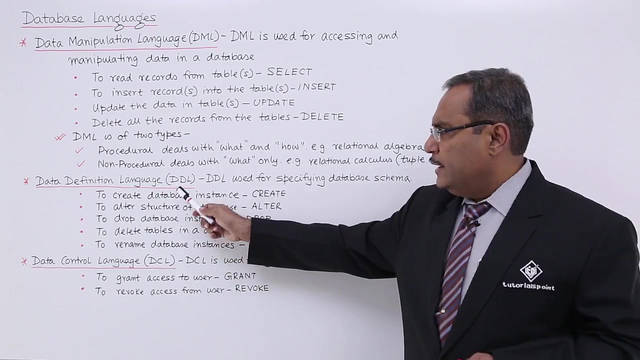 instances, that means you want to delete the table. In that case the command will be drop, Then delete. to delete tables in a database instance command will be truncate. To rename database instances, the command will be rename. The keyword will be rename. So these are the respective operations which you can carry out. 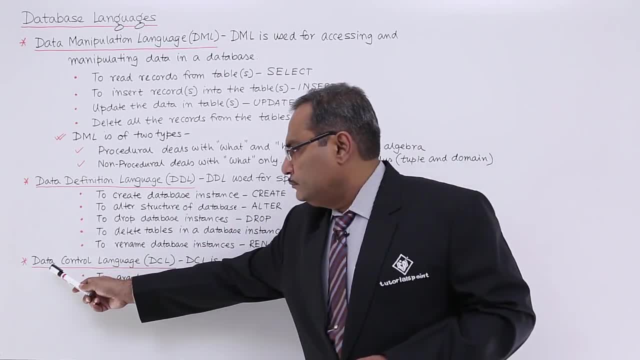 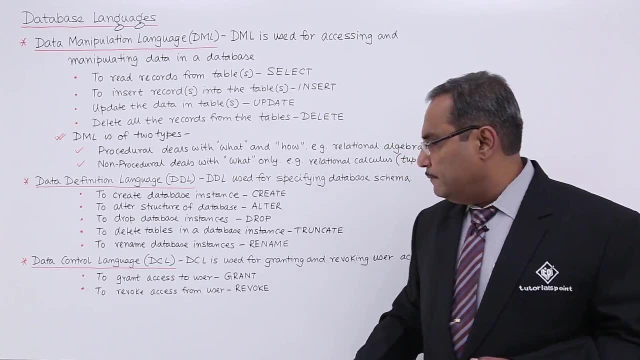 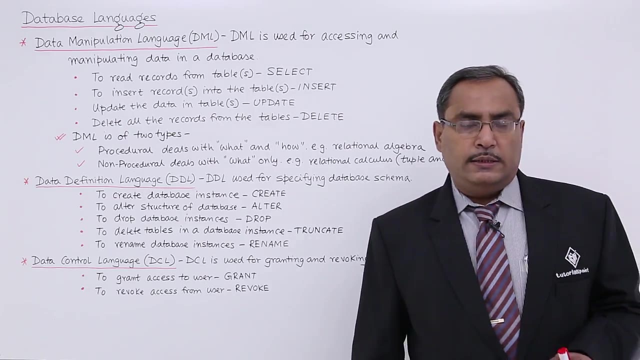 in our DDL. So now, data control language. What is the data control language? So, in short, it will be called as DCL. DCL is used for granting and revoking user access on the database. That means it will grant. Grant means you are giving permission to do something on the database. 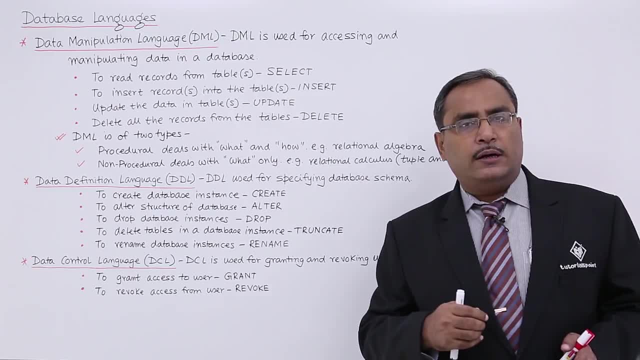 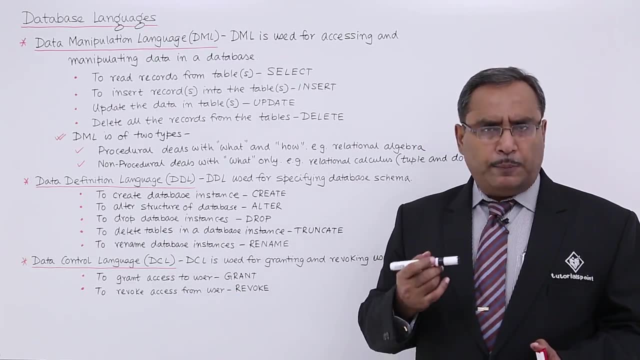 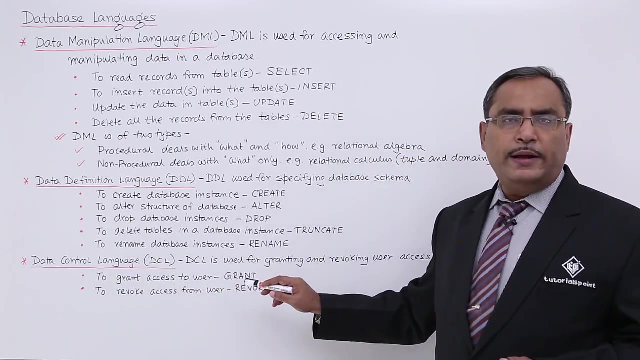 to one user and revoke means you are taking away the permission from the user. So to grant access to user. this access may be select, update, delete, insert and so on. So to this to grant access to user. here the command will be grant. To revoke access from user. you are taking away the access. 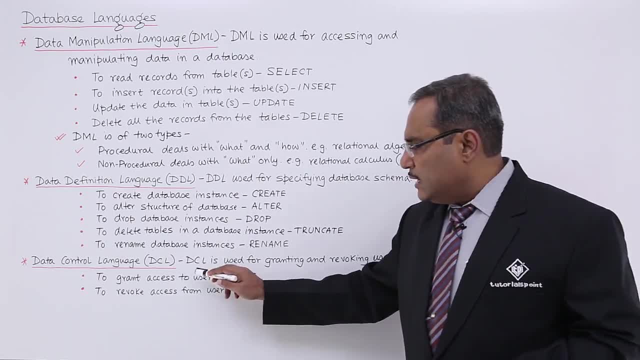 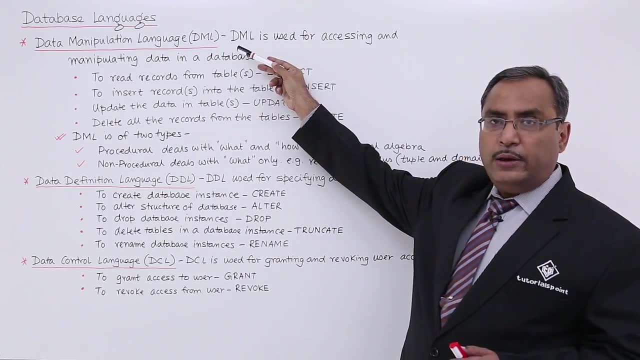 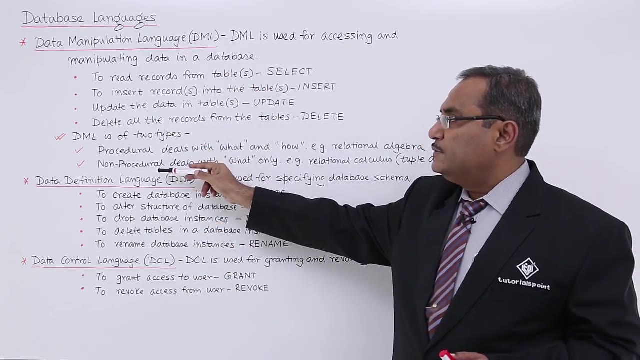 from the user, the command will be revoked. So these are coming under the category of data control language. So here you will be having this data manipulation language and data definition language. data control language, DML, will be of two types: procedural and non-procedural. So in this way, in this session, 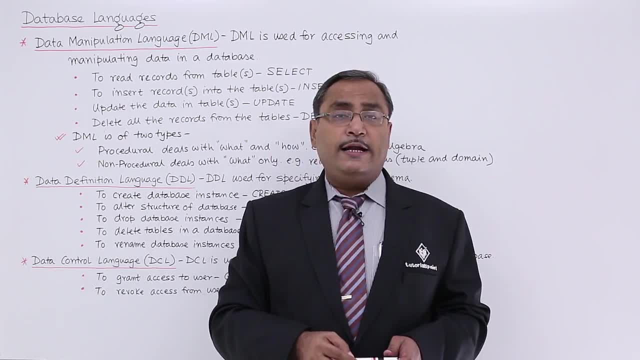 we have discussed what are the database languages and its different categories, with proper examples. Thanks for watching this video.